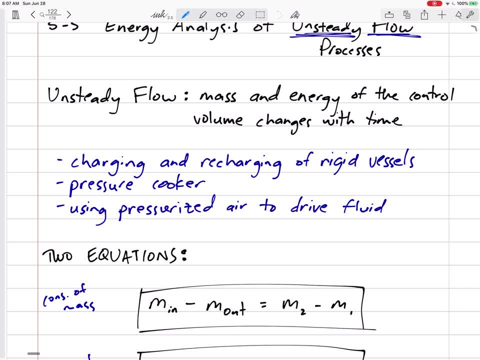 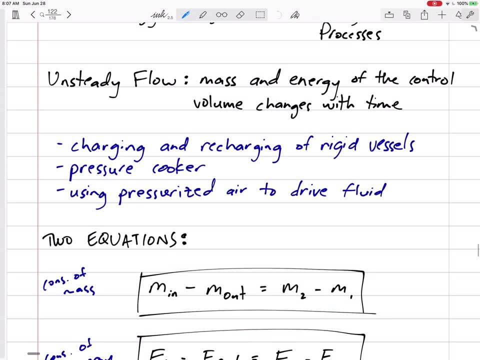 With this one. there are changes with time. There are initial and there are final, mass and energy. There's the initial situation and there's the final situation, in addition to the inlets and the outlets- and don't get them confused, We'll talk about that. So if we look at charging or 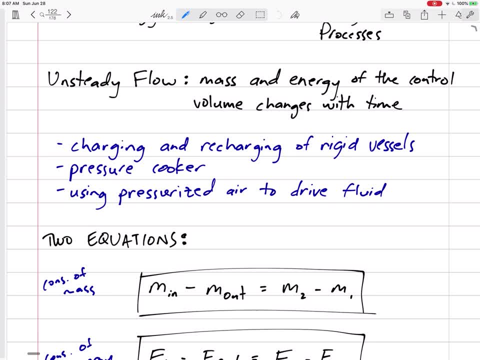 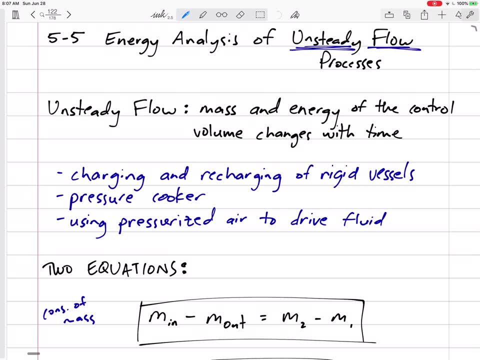 recharging of rigid vessels, pressure cookers using pressurized air to drive fluid. these are unsteady flow processes. When you see things where it starts with one amount of fluid and it ends an hour later- I don't know, 30 minutes later it ends. 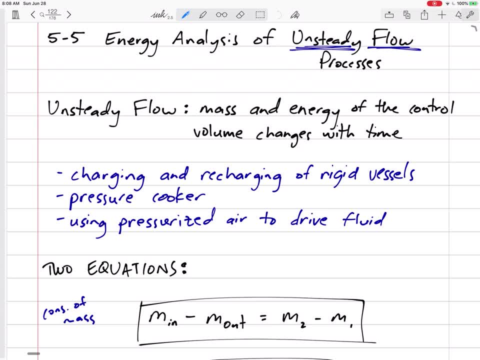 with a different amount of fluid. These are unsteady flow processes, So we can't use those equations. We can't use those steady flow equations, We can't use any of the shortcuts we have been taking earlier, But we still have two equations. We still have two equations. 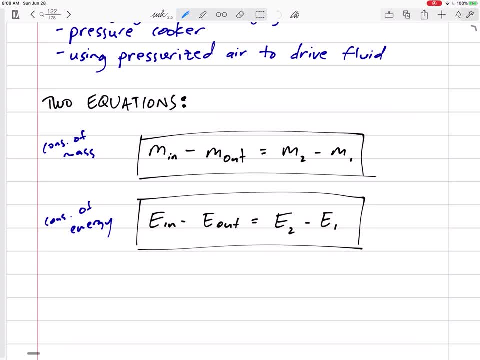 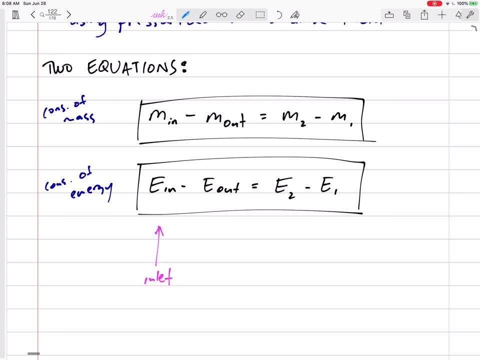 the mass, conservation of mass and conservation of energy. Now be careful here. All of this on the left-hand side is inlets and outlets. So this is the mass and the energy going in of the inlet mass and energy going out of the outlet. Do not get them confused with these. 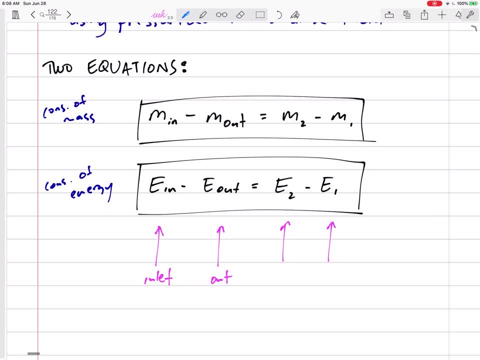 M2 and M1 or E2 and E1. And I have a bad habit, and the book does this too. Someone was back in the last section. for steady flow devices They say E2 and E1 are like inlets and outlets, but they kind of do a shortcut there because there's no change on the right-hand side. 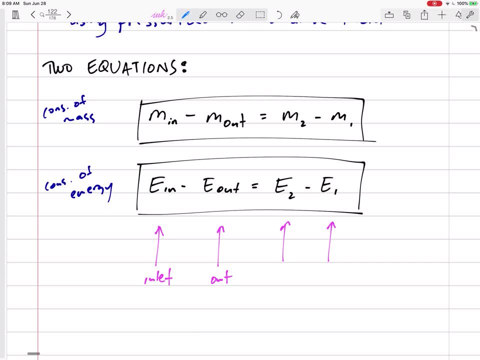 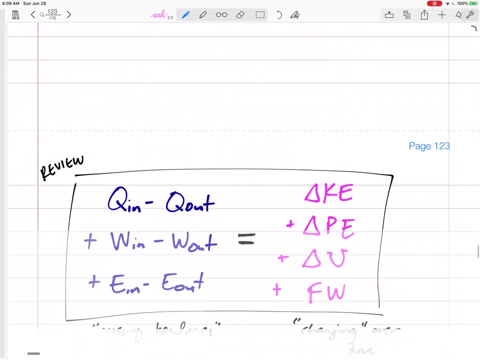 of the equation. They move the inlets and outlets to the other side of the equation and make them ones and twos. But here these are not inlets and outlets, These are final and initial, Final and initial. So let's just go to our remember. so this is review, because this is 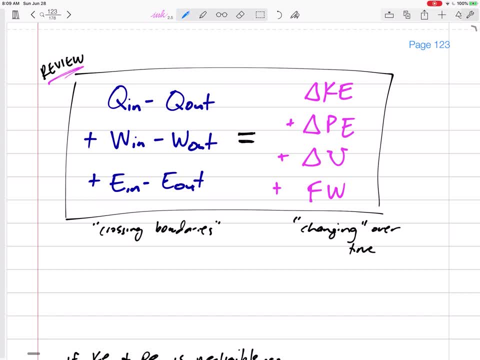 about the third or fourth time we've had this equation. This is our big conservation of energy equation, right. This is our big conservation of energy equation, right. The heat going in and out, the work going in and out, the fluid, the energy in. 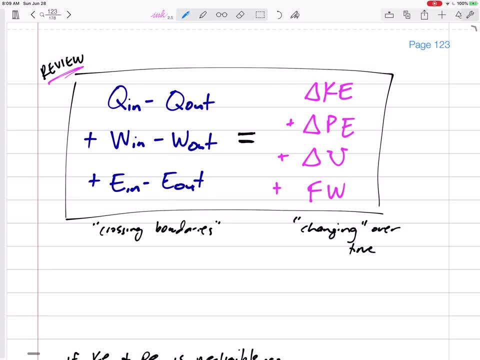 the fluid going in and out on the left-hand side equals the change in energy right, The change in kinetic energy, change in potential energy, change in U right, Total energy and flow work, And this is all changes over time, Whereas the left-hand side of the equation is crossing boundaries. So here's our big equation. 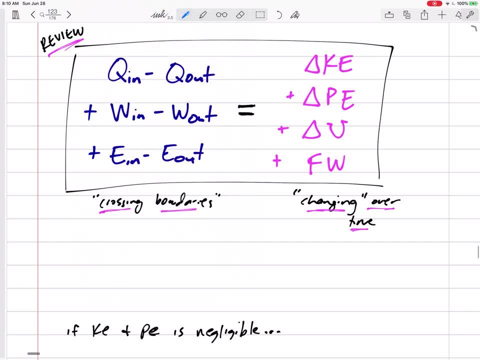 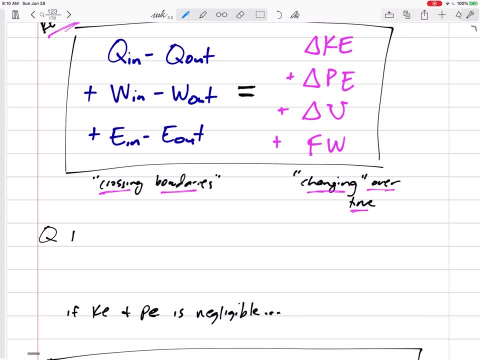 We've had this before, We've had this before, but we've always simplified it. So we're just not going to simplify it. So we need any heat transfer, plus any work, plus any. what is this? E? This is the energy in the fluid. So energy in the fluid going in and energy in the fluid going out. So 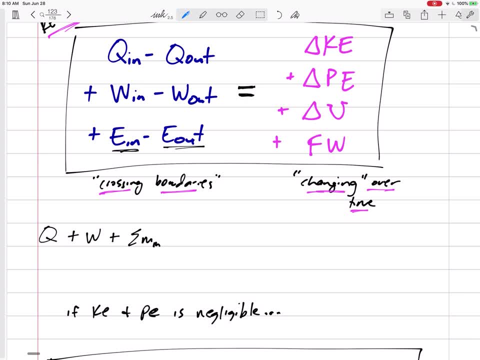 I'm gonna kind of sum all the mass in theta in minus all the mass out theta out. So think about how much mass came in times, how much energy was in that mass that was coming in. So this energy in the mass that was coming in, that would be H in plus kinetic energy in plus. 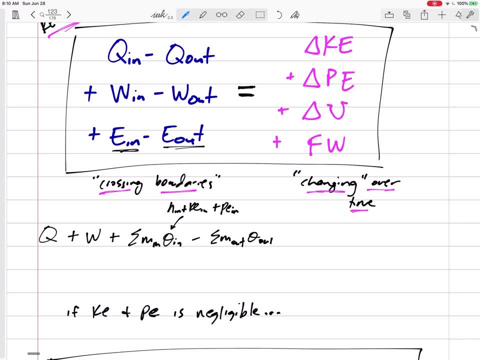 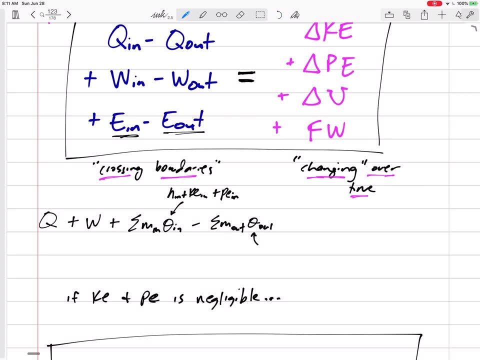 E potential energy ends right, This theta. just think about, okay, how much, how much mass was going out and how much energy was in that mass that was going out. So the energy in that mass that was going out is the H of the fluid going out, the kinetic energy of the fluid going out. 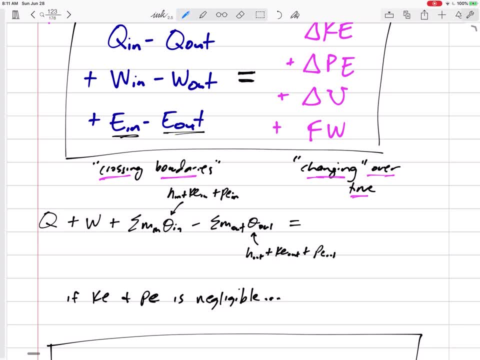 the potential energy of the fluid going out. All right, So all that- that's still just the left-hand side of the equation- equals the change in energy. So let's say the mass final energy final, minus the mass initial energy initial. All right, The mass. so just calculate how much mass. 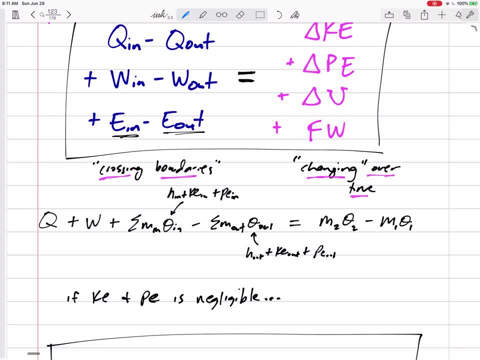 is in there at the end of the time, right At the end of the problem. how much mass was in there at the beginning of the problem? Now it may not give you the mass you know, just explicitly tell you the mass You might have to. 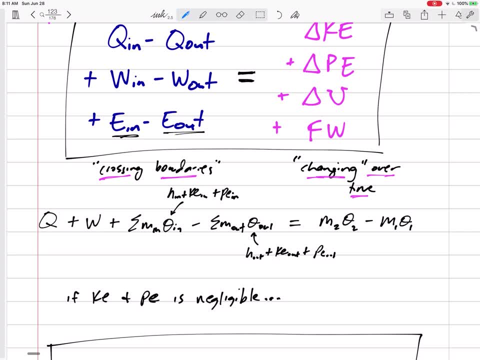 work that for that Might have to find the you know. if you know the volume and the specific volume, then then they tell you the mass. So some of these are not going to be just given on a silver platter. You have to work for these, All right. But this energy in the fluid, 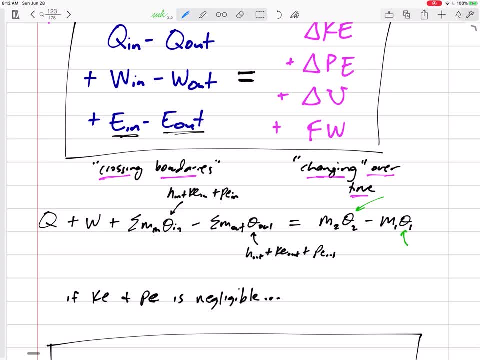 initially an energy in the fluid. Finally, this is: it could be H and K? E and P E, or U and K E and P E, U plus K, E plus P E. When should we use H? When should we use U? Well, use H if it is a constant. 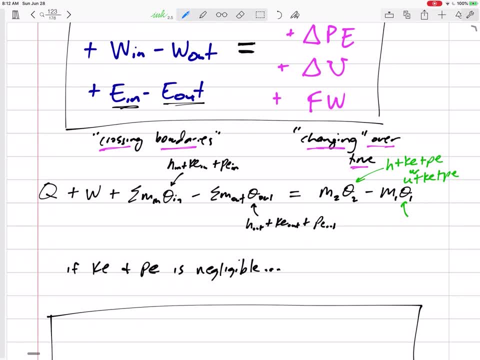 pressure process that the volume is changing. right. Use H if it's a constant pressure volume change process, because then that H we don't have to calculate boundary layer. We use U if it is not a constant pressure process. We use U if it's a rigid. 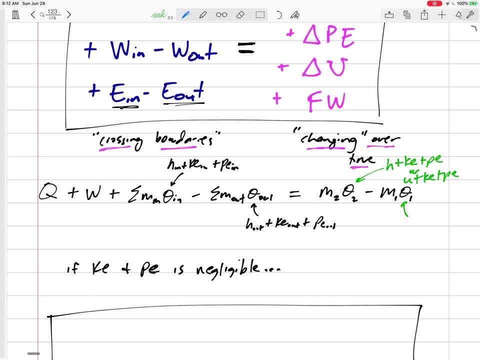 Tank And if it's a rigid tank we don't have to calculate boundary work. but do be careful. I think there are some problems where, if it's not a constant pressure or not a constant volume process, if it's, if it's some other weird process, what would we do? We would use U and we. 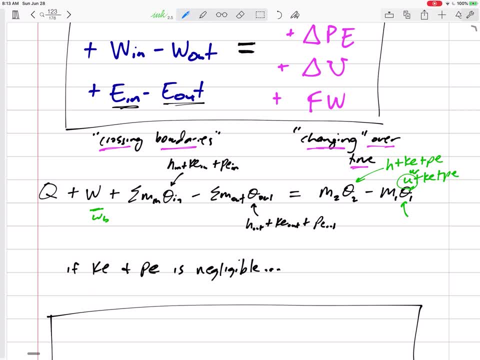 would still calculate some boundary work here on the left-hand side of our equation. So so here, this is the. you know, this is all the final H, the final kinetic energy, final potential energy, And this is the, the initial. 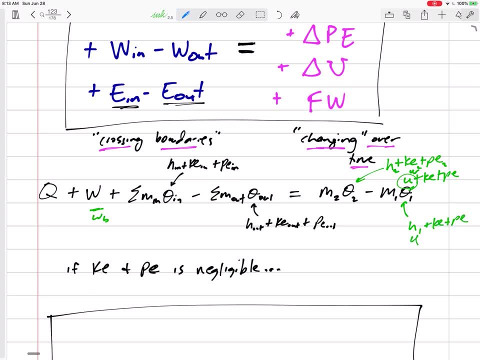 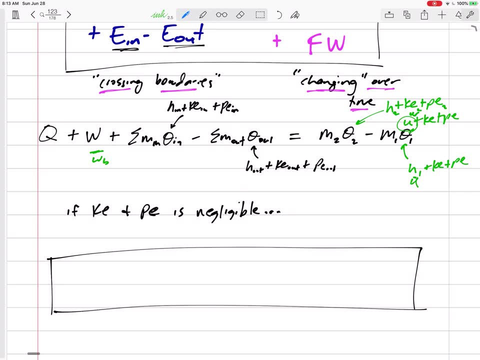 H: kinetic energy plus potential energy. Now this might be U, H or U. Okay, Many times the kinetic energy and potential energy is negligible. We did a problem- I don't know if you saw notice. we did a problem where we saw that even a change in height of a hundred meters only changed. 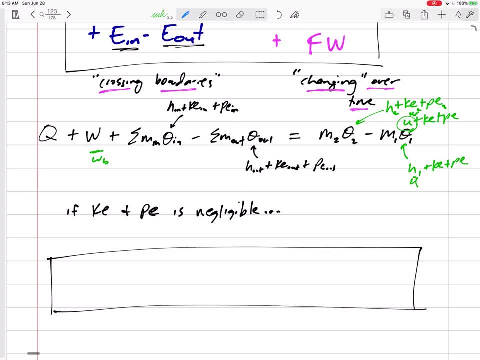 the energy by one kilojoule per kilogram And also a change in velocity of or a velocity of 45 meters per second. only changed um the energy one kilojoule per kilogram, And so if we're looking at thousands, you know. 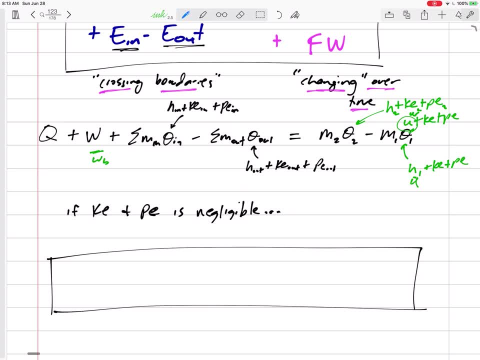 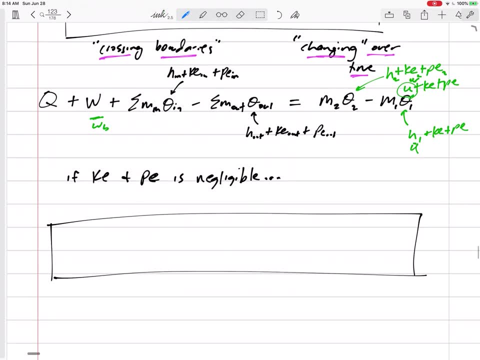 2000,. 3000 kilojoules per kilogram, then most of the time that kinetic energy and potential energy is negligible, Most of the time they don't tell us the kinetic energy or potential energy, So so we can assume it's negligible. So, uh, if it is negligible, so either they don't tell you.